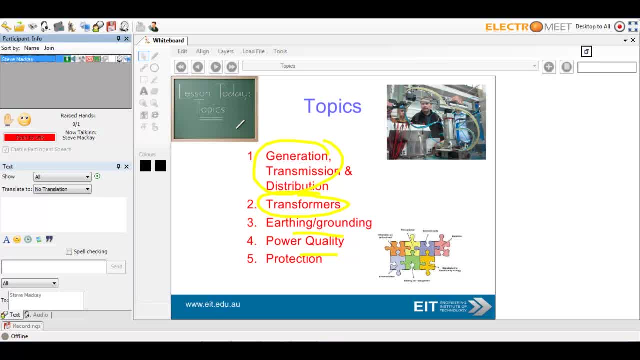 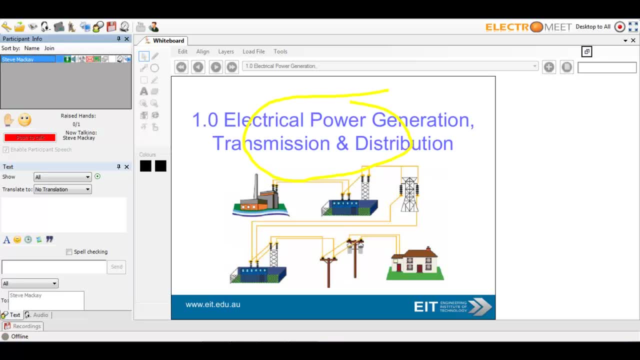 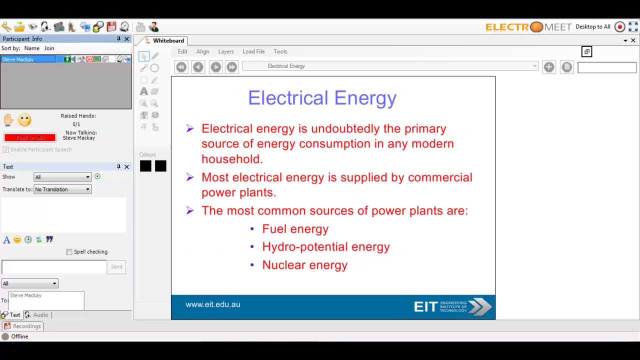 distribution, transformers, earth and grounding power quality protection. So first thing is electrical power distribution, generation and transmission. Here's your generation, here's your transmission and here's your distribution at the end of the road towards the houses. Energy conversion is the critical part of the whole process. 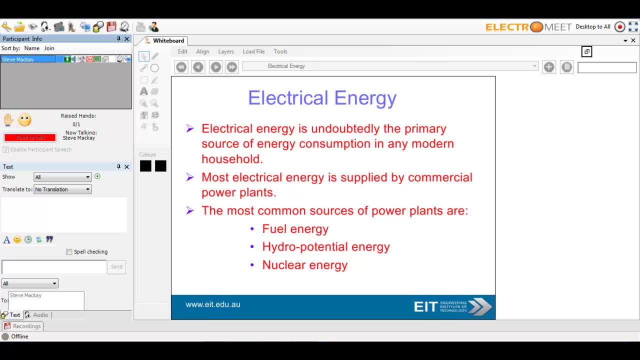 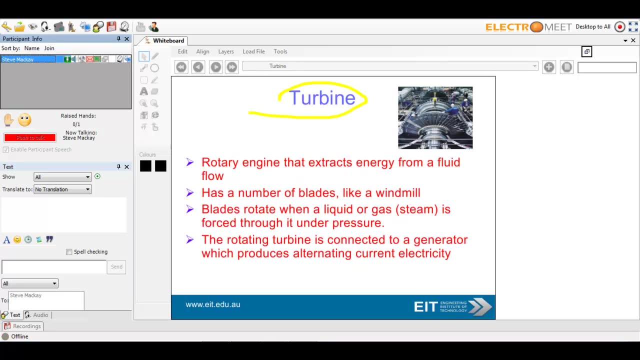 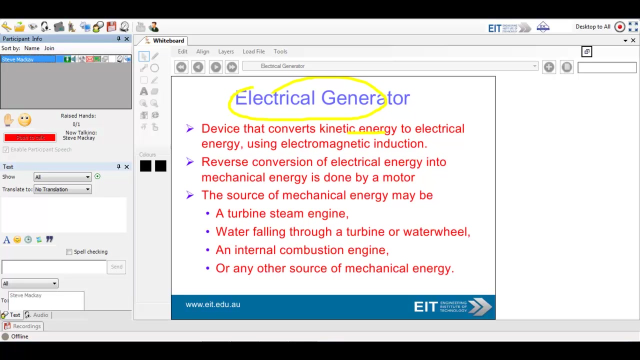 What this means is that we take mechanical engineering or chemical materials converted into mechanical movement and then convert it back into electrical energy, which is probably the most flexible form of energy to work with, Using a turbine, for example. Electrical generator will then convert the kinetic energy half e m v squared- to electrical engineering energy. 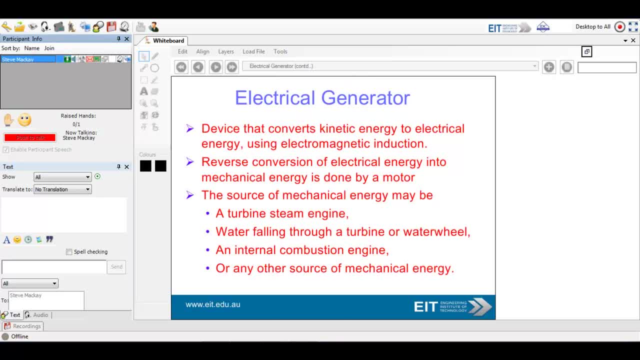 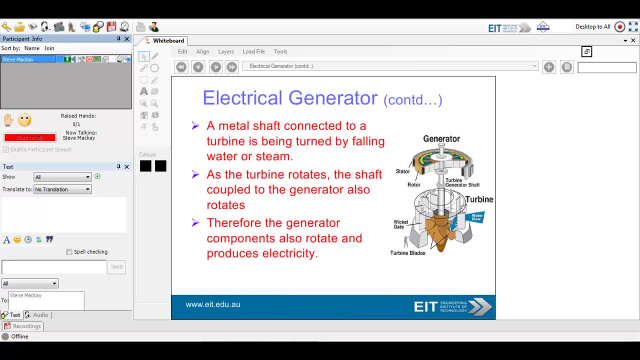 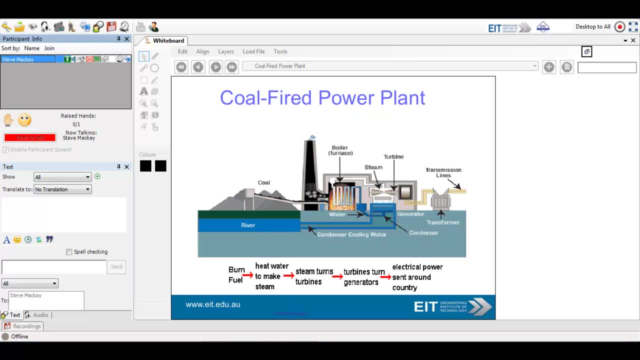 using electromagnetic induction. So basically, this is an electrical generator, a power station, And the idea is that we have a coal-fired power plant. You've got your coal, coal burning, boiler, steam generation, the turbine and then eventually on the transmission lines. 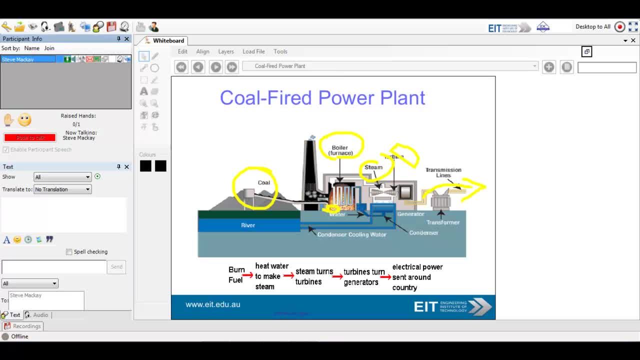 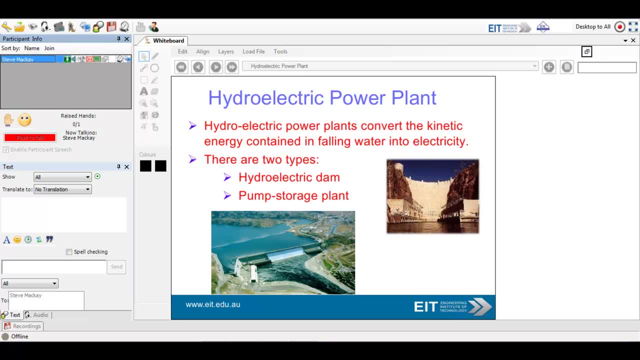 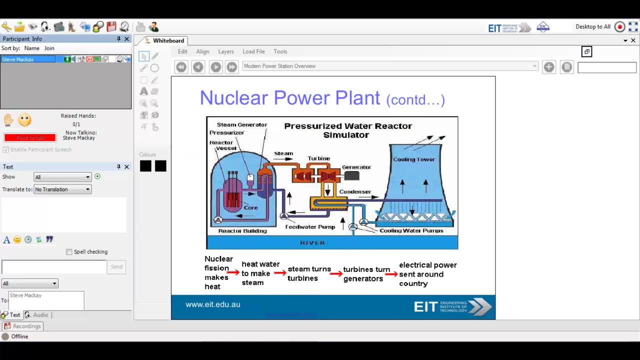 out to the particular industrial site or household, And this process is repeated in the combustion turbine plant. Here's your hydroelectric plant, Slightly different: where you've got water, Obviously no droughts required. Nuclear power plant's another one. Here's a summary of a power station. 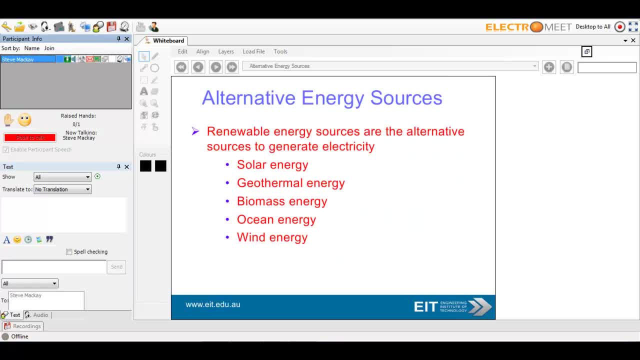 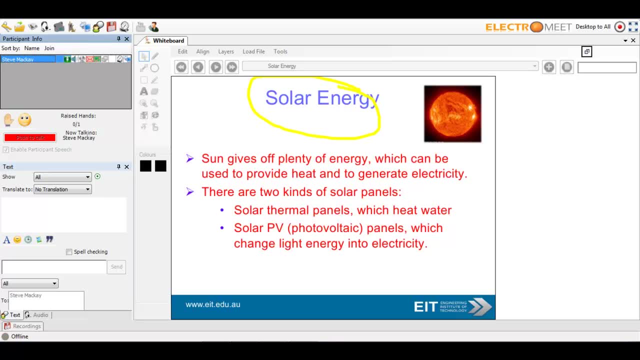 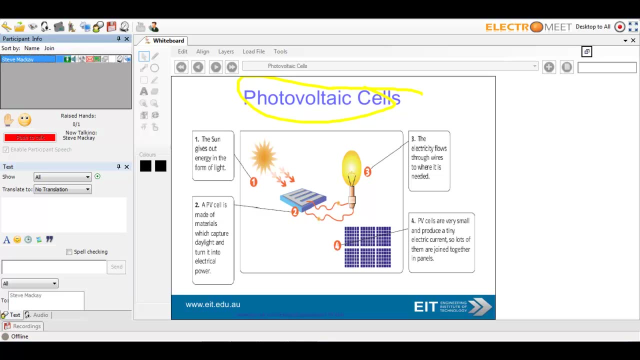 overview. If you want to stop at any of these slides, just pause the presentation and you can see quite quickly what's going on. Solar energy is obviously very appealing today because it's emission free. Photovoltaic cells are rapidly falling in price, So they can make quite a big contribution And, as someone said the other day, it's a 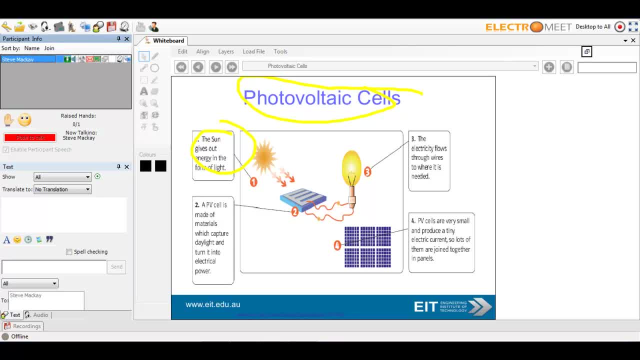 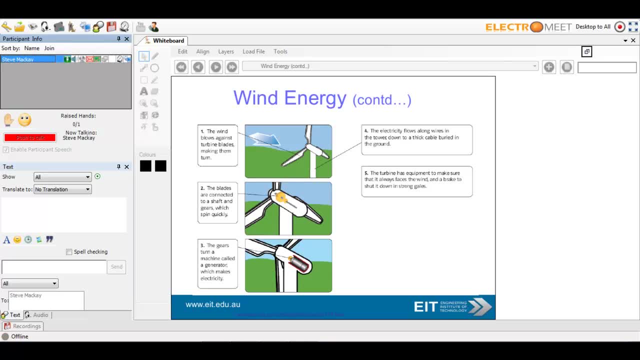 fusion source providing power wirelessly over millions of miles. Quite amazing. Wind energy is the other form of power. Unfortunately, wind energy does have a few challenges with environmental pollution. in terms of your view of the household or the rural guys, Probably a little bit compromised. 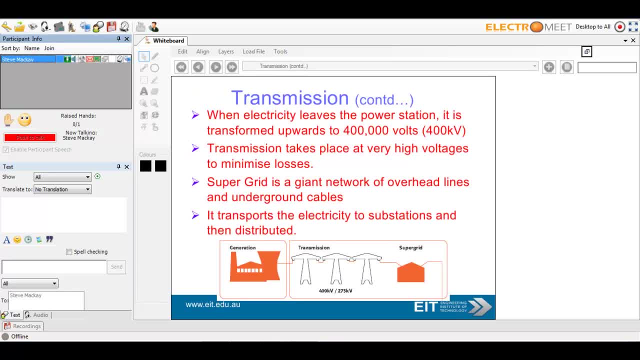 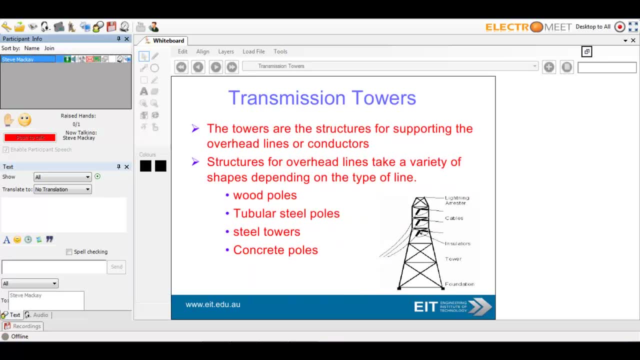 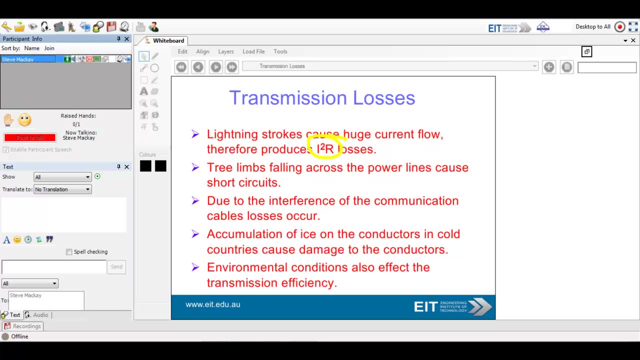 Transmission of energy. Transmission of energy, Transmission of power, is the next thing, Typically at 400 kilovolts and very high voltages to minimize the I squared R losses. Transmission towers are critical. So it's quite a big, strong mechanical engineering component there And you can imagine what happens with power lines. 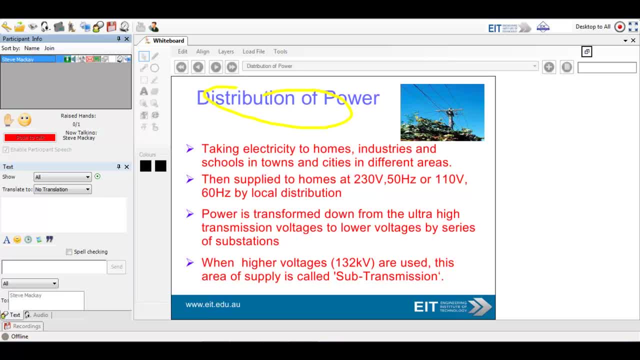 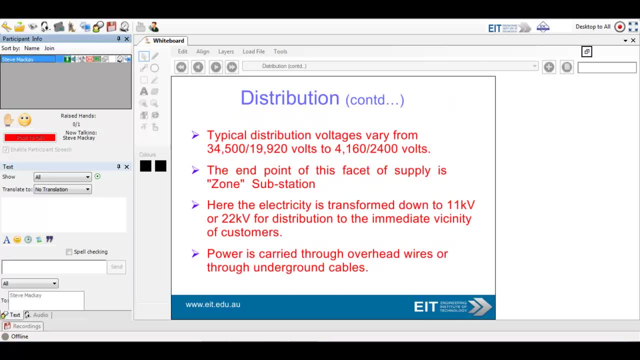 during snow, ice storms. Then we have distribution of power: Takes the power to homes at 230 volts. 230 volts is probably the standard used today. It used to be 240 or 250 volts, indeed, in Western Australia down to 220 volts in the UK, Which? 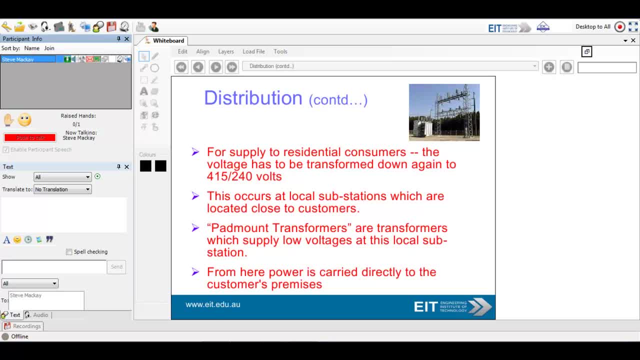 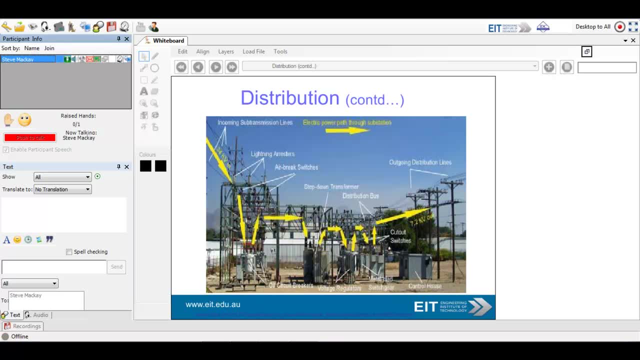 we've standardized on 230 volts. We have a substation that will take the power and convert the transmission sub-transmission lines down to distribution lines. here, as you can see. You can see also here that you've got your, obviously, your transformers, Oil circuit breakers, Those you'd be able to see. 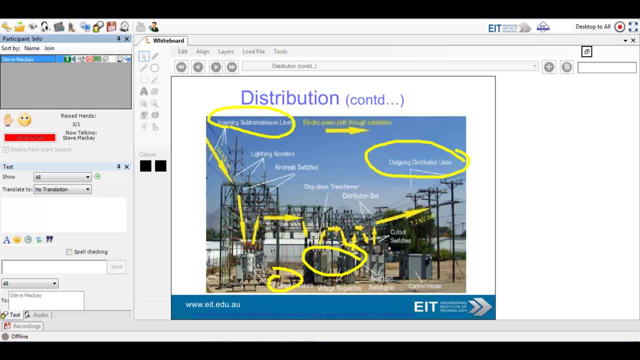 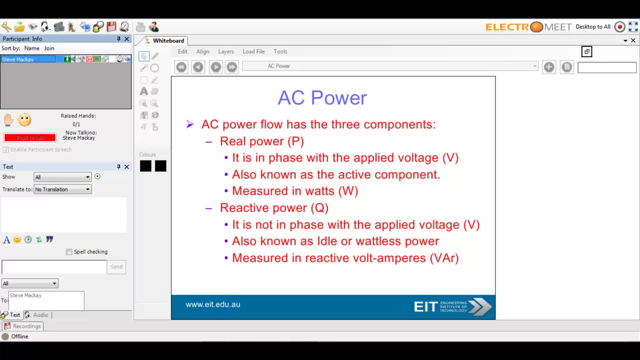 here, These voltage regulators etc. And we push the power out at a considerably lower voltage than when it comes in at 400 kV or lower. AC power is three components: The real power, Reactive power. Obviously it's reactive power is probably not useful in terms of providing power to the power supply, But it's a very 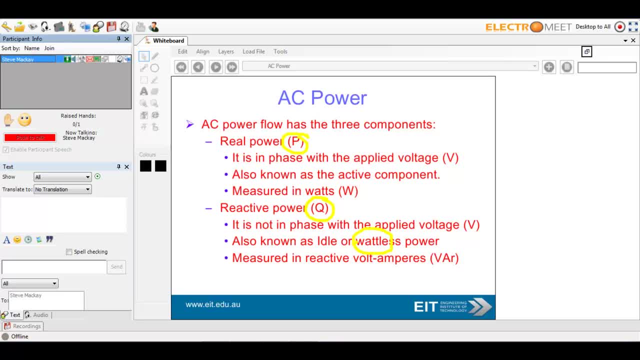 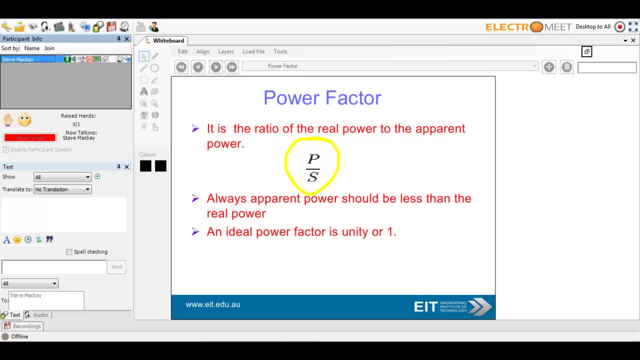 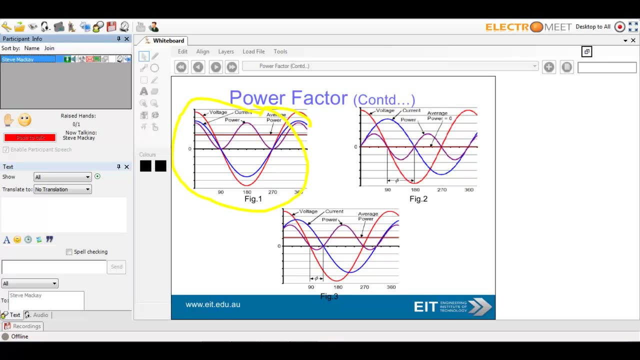 important component in terms of providing energy for moving stuff. It's a real power that matters And this goes together with the concept of power factor- Very important- And ideal power factor is one Very hard to realize that. And ideal power factor means the voltages and currents are completely aligned with each. 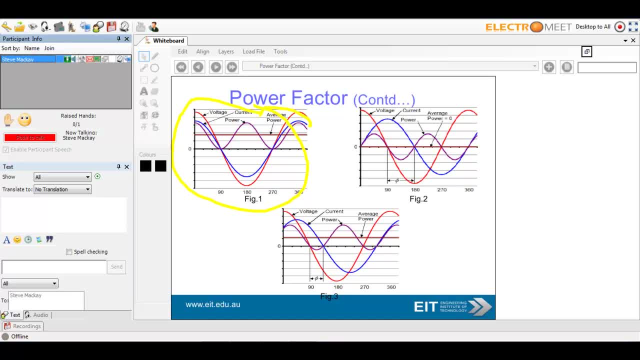 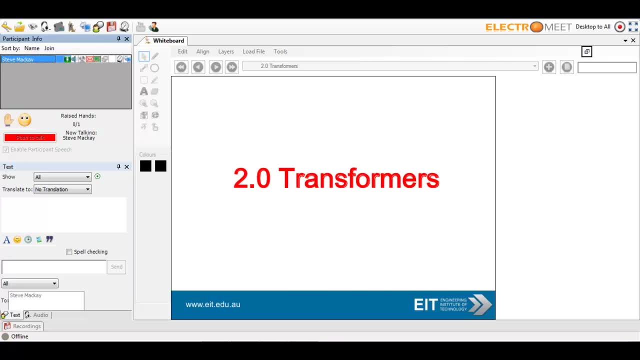 other. So voltage and current, there's no shift. If you look at this one here, you've got your voltage and current waveform shifted And of course your power factor will be less than one. Transformers are obviously very important to raise or lower voltages. Here's a typical. 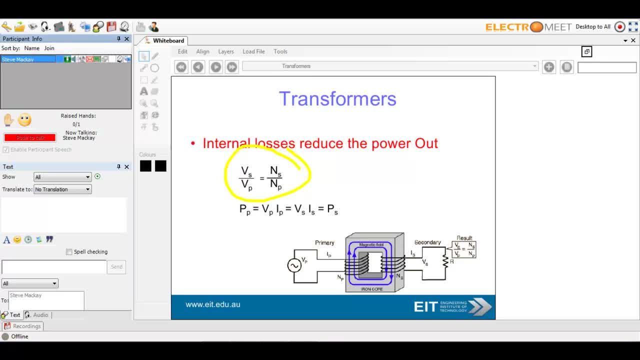 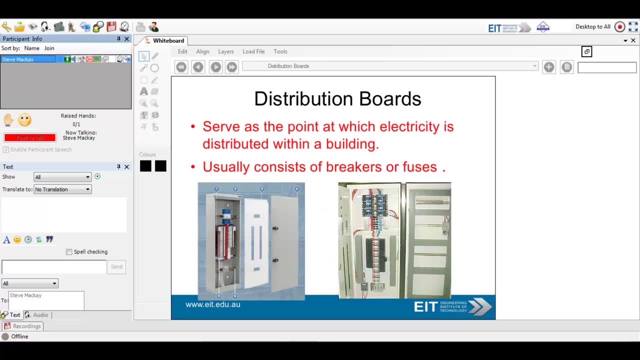 formula V secondary over V- primary equals number of turns of secondary over number of turns of primary. So this is the fundamental building block of a transformer- Very simplified diagram. of course, Power transformers are very important And obviously And distribution boards to distribute the power. 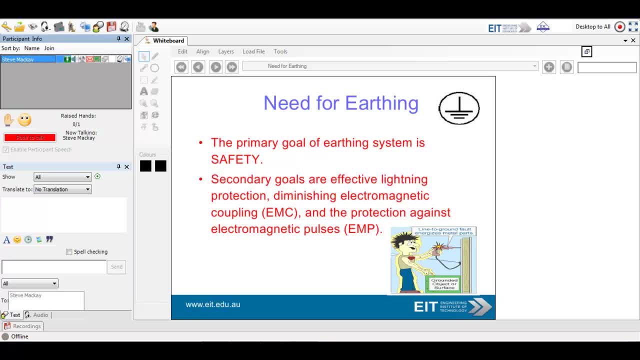 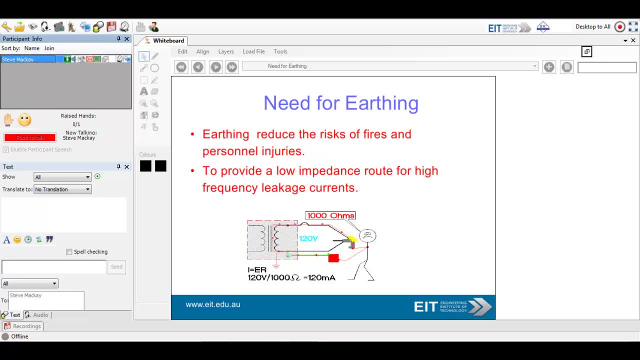 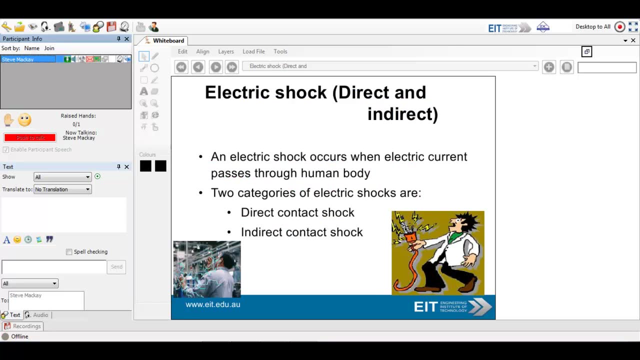 Earthing, grounding, is another very important issue. It's all about safety. And then you've got earthing here, very important Low impedance route for high frequency leakage currents, And obviously the idea is that you earthing is very important to avoid electric shocks. 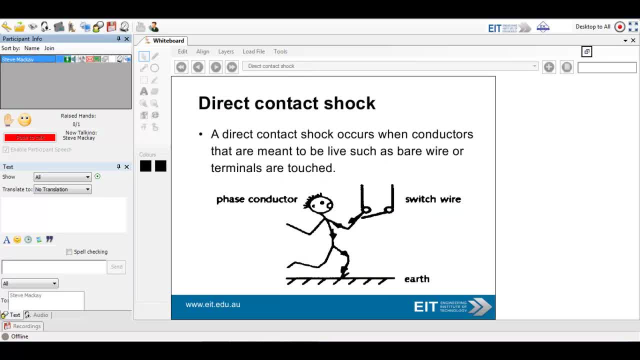 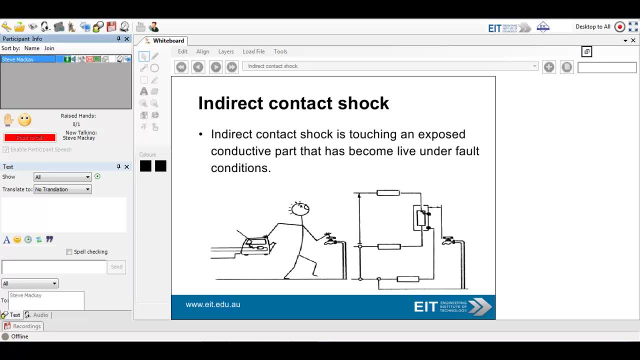 either direct or indirect And, of course, if you're going to work with your power supply, you've got to be aware of the difference in current Direct contact. is obviously you touching something which obviously could be very dangerous, or indirect? is you touching an exposed conductive part to become live under fault conditions? 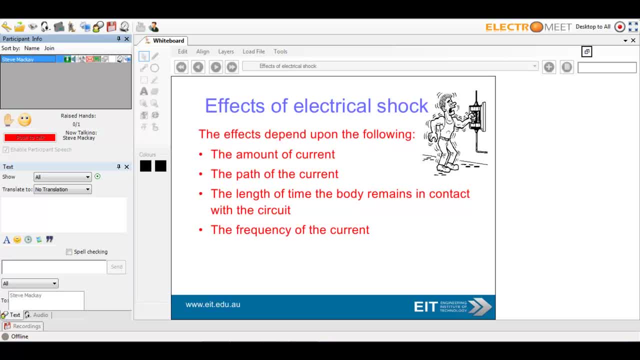 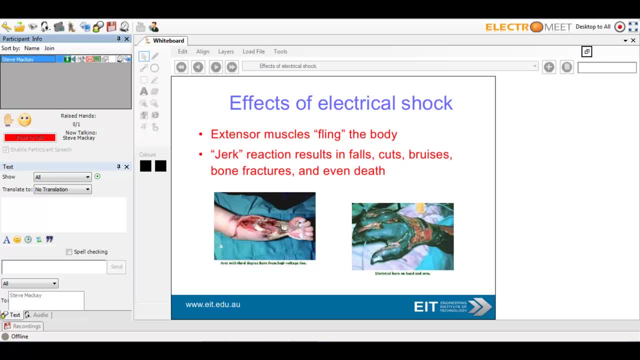 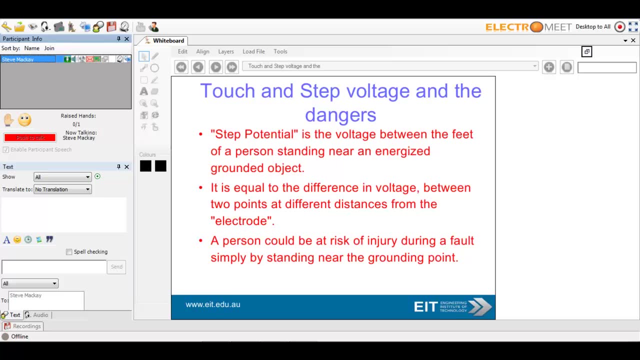 Obviously either situation is not good and obviously the amount of current going through your body will impact on your heart and, of course, cause problems. Some very nasty pictures here of injuries caused and obviously the other one is arc flash, which can be pretty bad Touch and step voltage- very important to understand the difference. 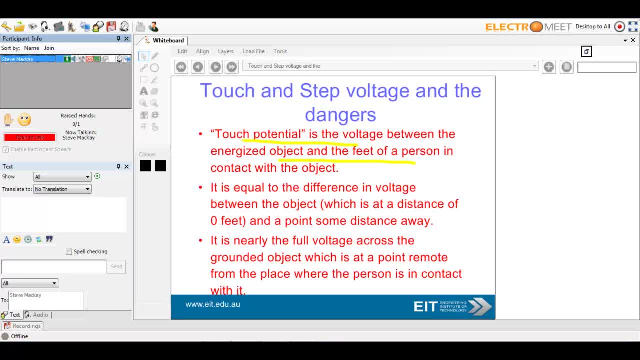 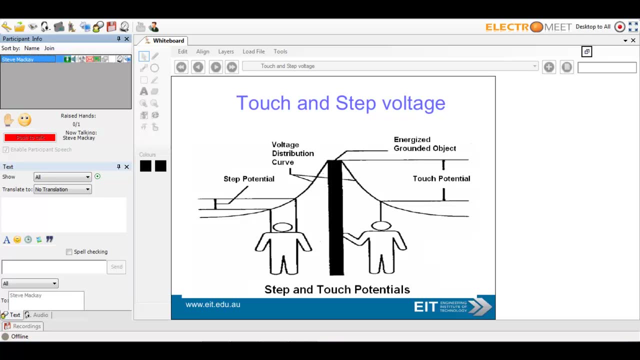 A touch potential is a voltage between an energized object and the feet of the person in contact with the object. So it's a voltage difference between the object and a point some distance away. So touch. here is an example Touch potential. You can see here he's touching something. 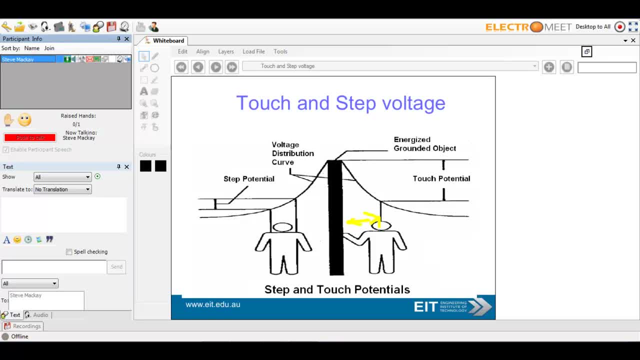 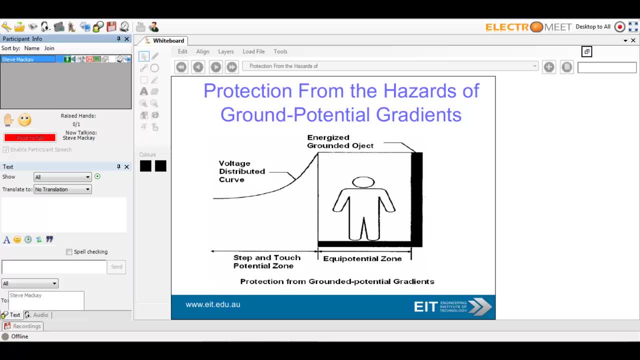 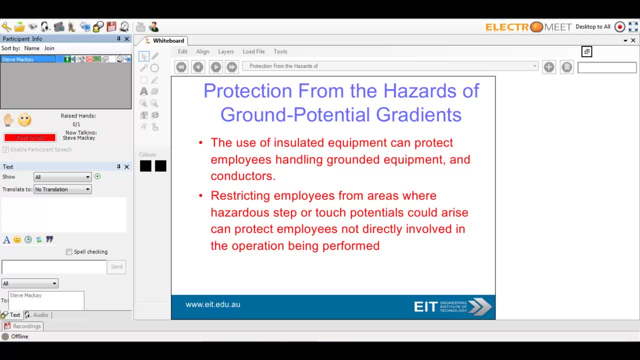 So that's the voltage across there And step potential is the voltage between the body. So obviously the idea is to avoid everything being grounded or earthed. Earthing is a term used in the IEC, International Electrotechnical Commission- world, which is European, Pacific, Asia Pacific and Africa. 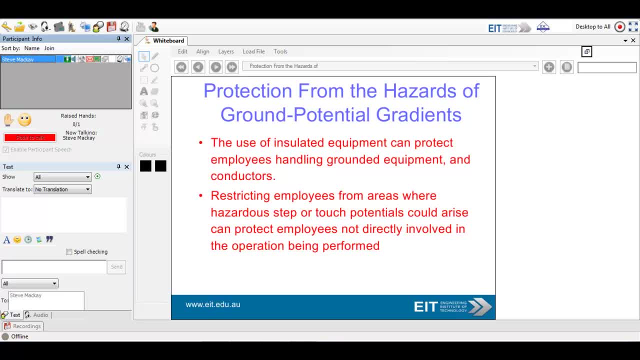 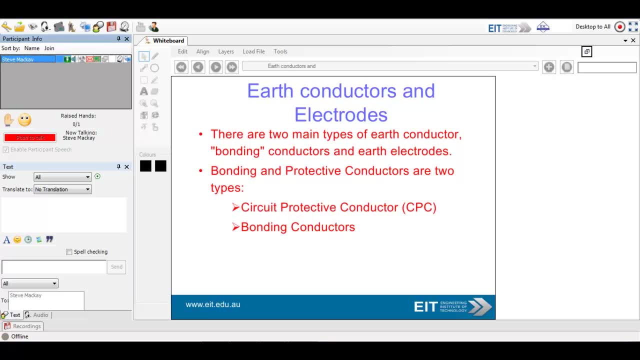 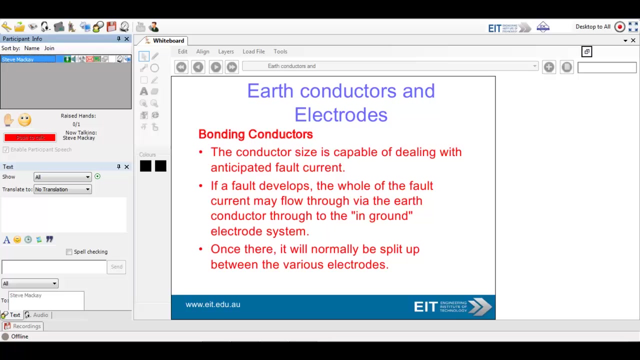 Right And earthing is often used is a key term used in North America, Canada and the States, And the other issues are earth conductors, electrodes, two types of conductors, bonding to tie conductors together. dealing with fault currents, Earth electrodes go into the ground. 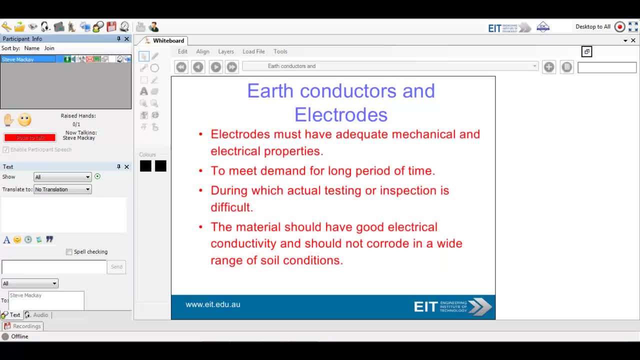 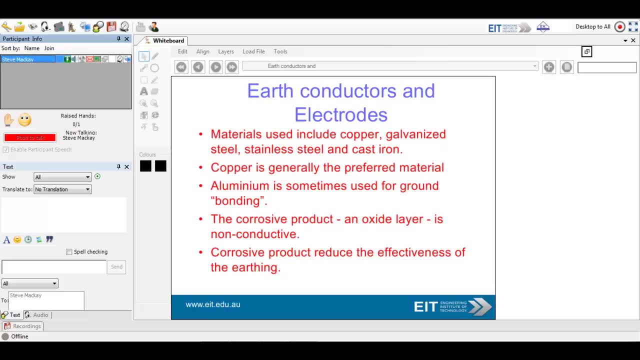 Right. Very important to carry significant amounts of current as well, Copper is often the preferred material. Be very careful with corrosion of some of the less noble metals when using as earth conductors. So you can have vertical rods or plates and horizontal conductors. 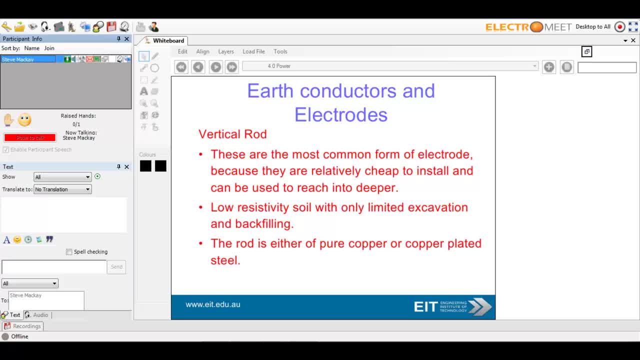 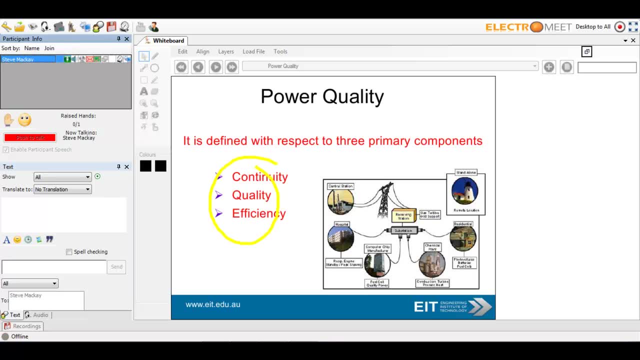 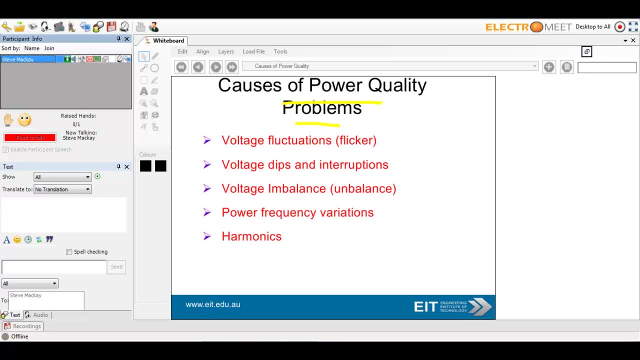 Most of them are vertical rods, Vertical rods And the power quality is the other important issue. Basically, there are three primary components- Continuity, quality and efficiency- And there's a whole reason of different quality problems: Fluctuations, flicker dips and interruptions, imbalance between phases, frequency variations from 50 Hz, for example. 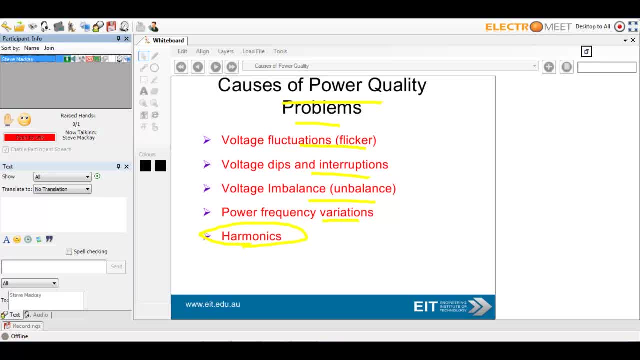 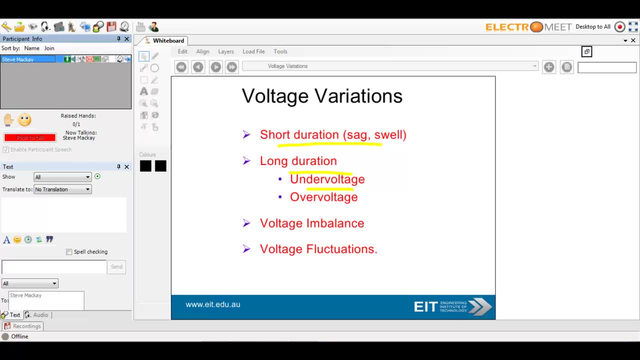 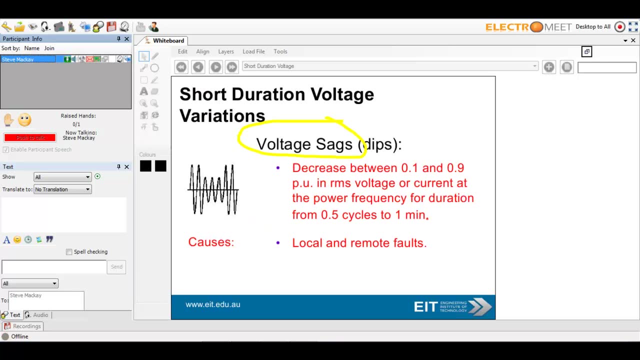 Or in America 60 Hz, and obviously harmonics caused by variable speed drives. So short durations, the sag swell. Long duration under voltage over voltage, Voltage imbalance, voltage fluctuations, Voltage fluctuations. Here's an example of voltage sag. 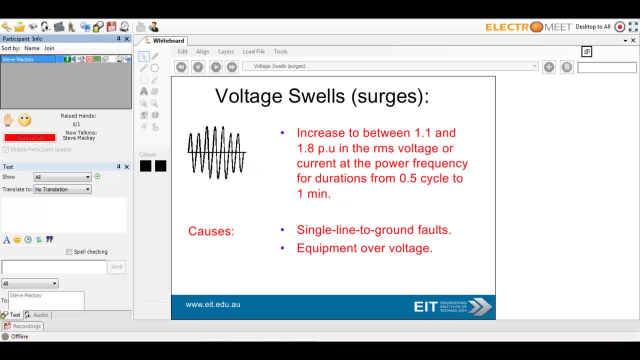 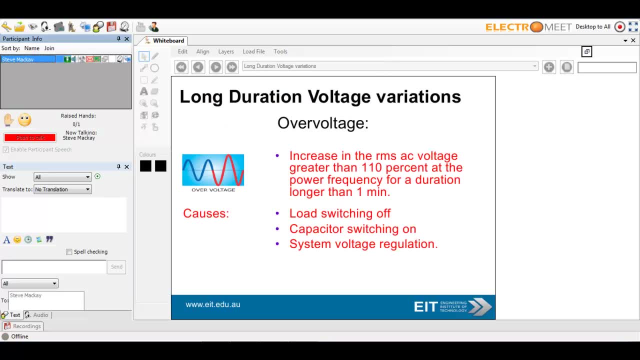 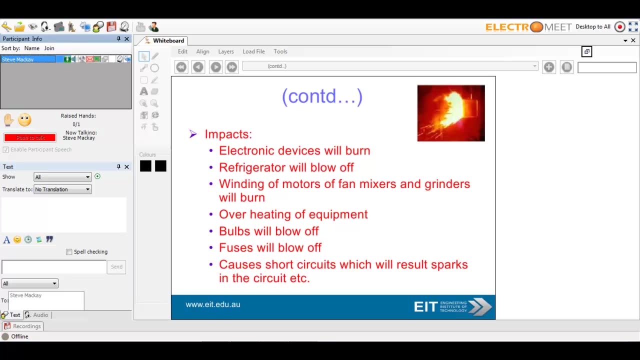 I'm not going to go into too much detail here, But here are the different types And obviously it could be enormous damage to your equipment. Voltage swells or surges, Long duration, voltage variations over voltage, It can cause problems with your especially electronic equipment under voltages. 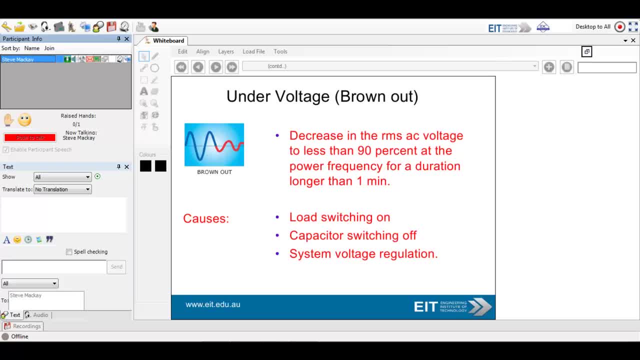 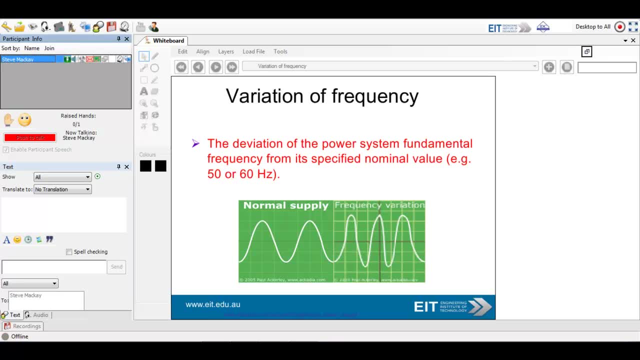 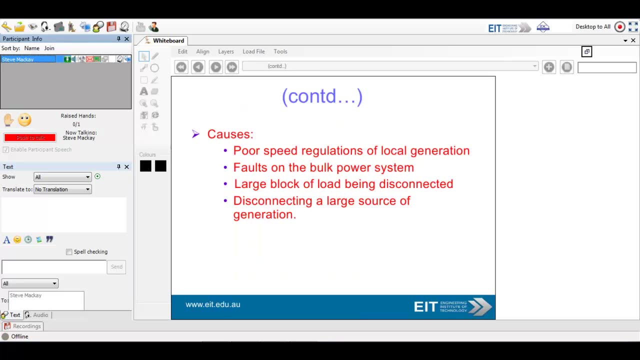 When a generator can't really provide the power required. So you generally have under voltage Or they drop the frequency as well. That's another trick. It means people, the devices, use less power. Variation of frequency: 50 Hz. It's very important to keep the average to 50 Hz at all times. 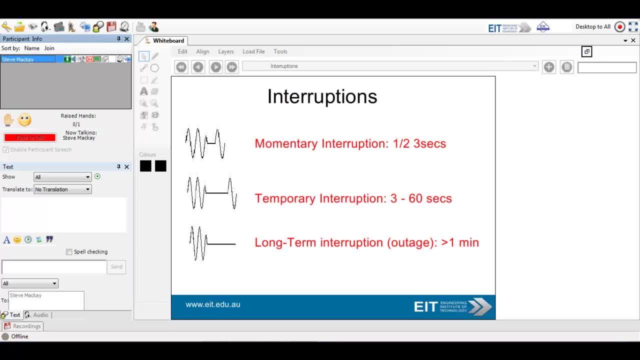 Interruptions: half a second. three seconds. Momentary interruption. Three to 60 seconds is temporary interruption. Long term interruption is greater than long term. Momentary interruption is greater than one minute. Those are the sort of definitions that are used. 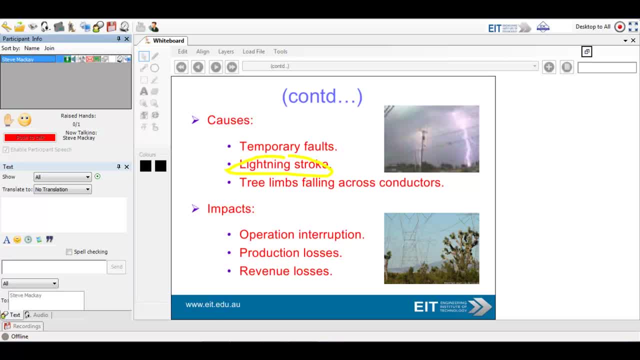 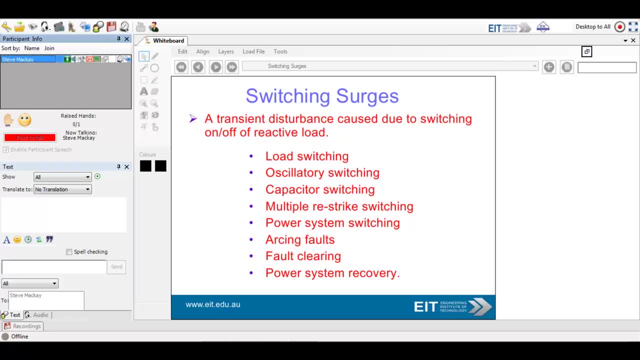 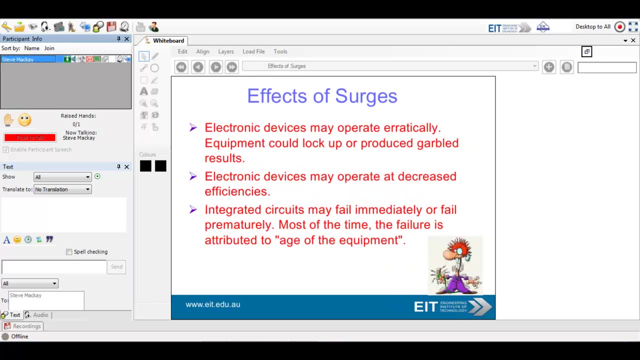 Could be caused by lightning stroke, for example, Or other particular issues: Tree limbs, Surge, Surge protection is very important, Especially in lightning prone areas: Switching surges, Lightning surges- It's obviously a big problem, And this leads us on to the next topic. 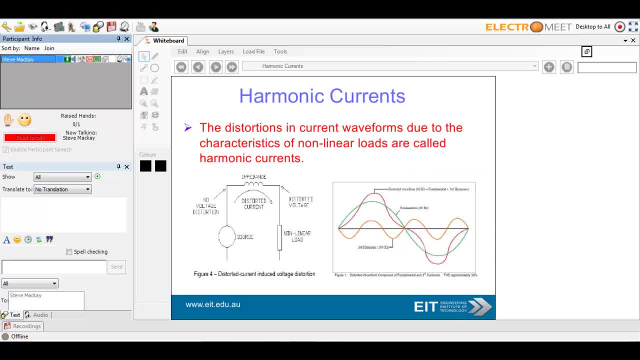 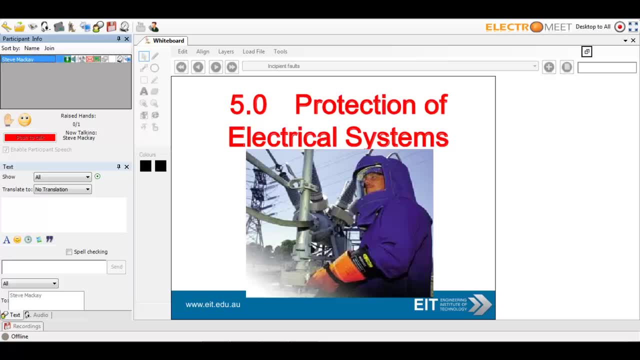 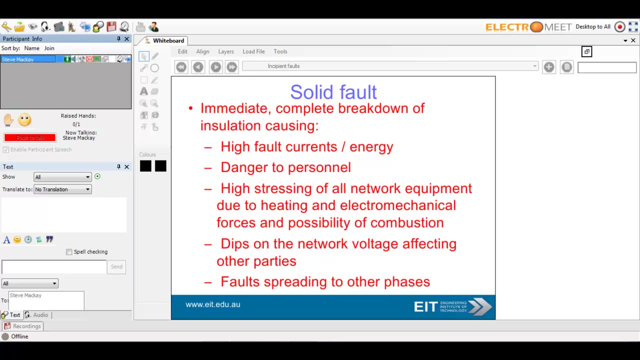 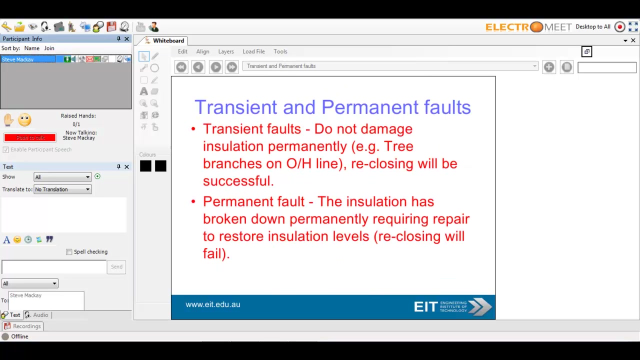 Which, of course, besides lightning arresters, is protection And Protection of your electrical systems. Just to briefly talk about protection, You can have a solid fault or an incipient fault, So the idea is that transient faults do not damage insulation permanently. 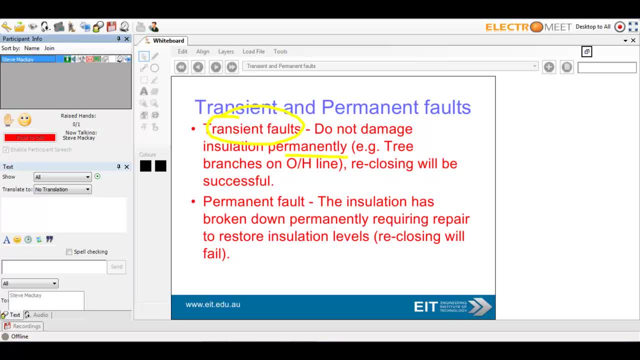 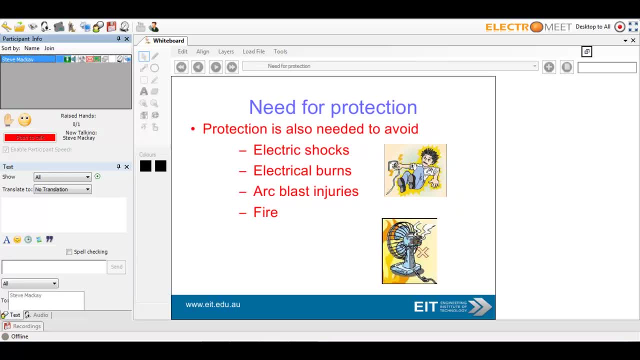 It's quick, And a permanent fault obviously is something a bit more long term. So the insulation of your cable, which is paper based from 50, 80 years ago, has destroyed itself. So you've got a permanent condition, Permanent fault condition which could be expensive. 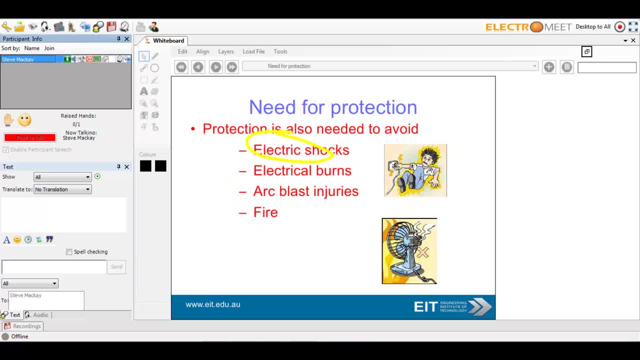 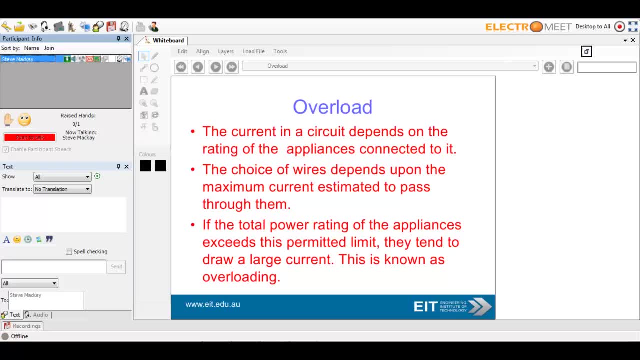 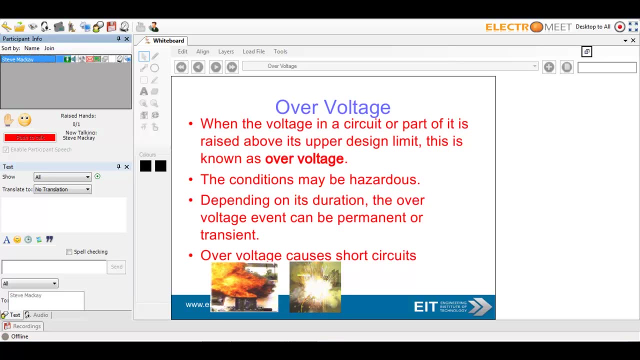 Need for protection. Really important: Prevent electric shocks, Electric burns, Arc flash, Arc flash or arc blast And fire. Overload protection, Protect from hazards, Overvoltage, So protection Overcurrent is another one Exceeds the amperage rating. 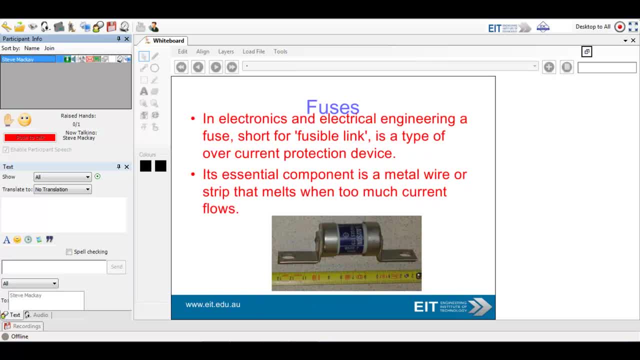 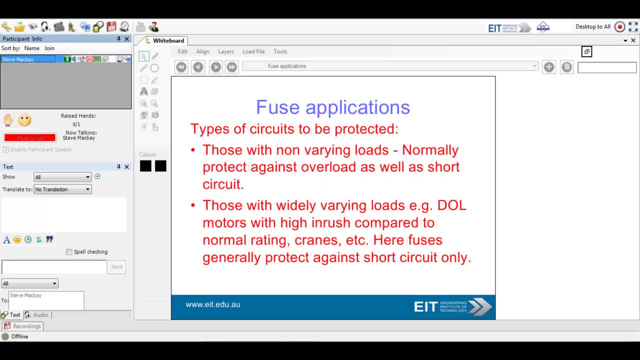 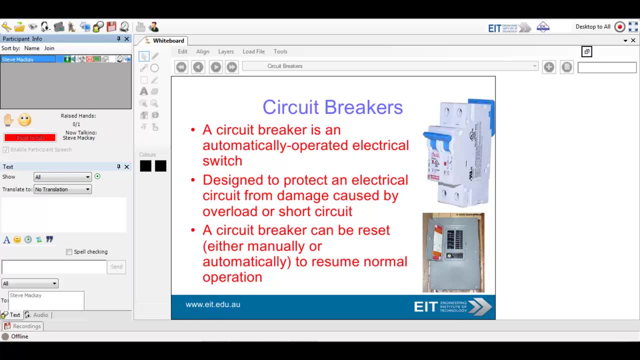 You obviously want to protect your motors and current and your conductors, And fuses are often used Or relays, So fuses could be quite important. Circuit breakers are also very important, Probably more so than fuses Automatically operated. 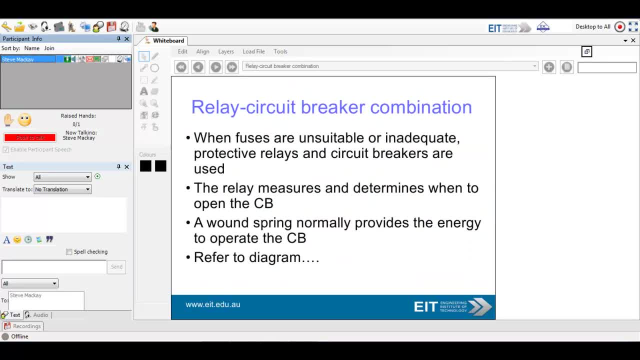 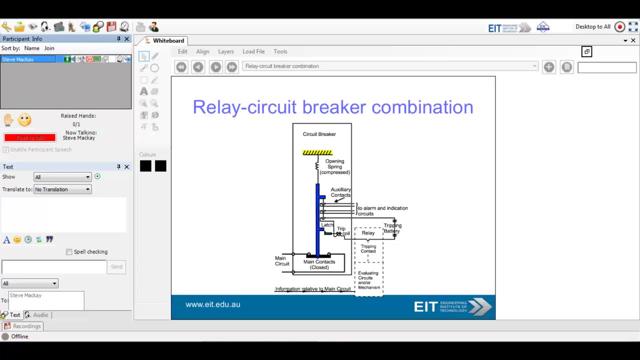 And you can generally reset the circuit breaker. So you have a relay-circuit breaker combination. Relays and circuit breakers are used. Relay detects when to open the circuit breaker and sends a signal to break the circuit. So circuit breakers are very important.